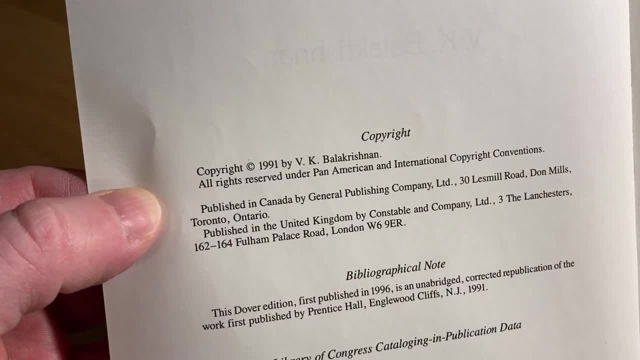 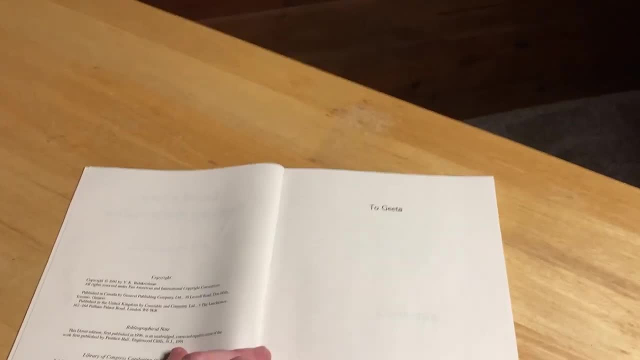 you can see what it covers. Here's the copyright: 1991 by V K Balakrishnan. Cool, Yeah, and so this is a book you can use to learn discrete math on your own or if you're in a class. 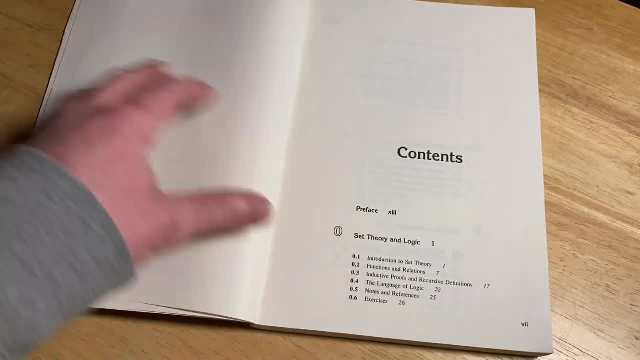 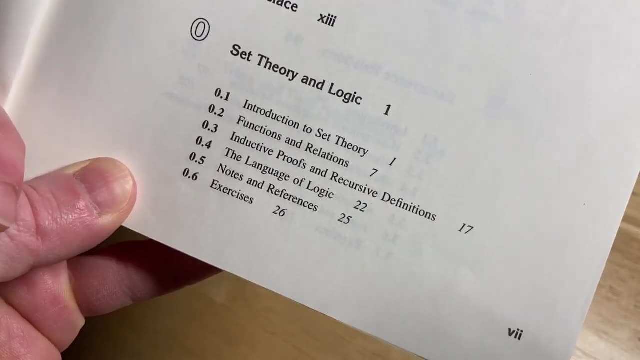 I do think this serves as a fairly decent supplement. Again, no discrete math book is perfect. This one is really affordable, though. That's why I wanted to make the video on this one. It's not super expensive because it's a Dover book which is a reprint, so it's 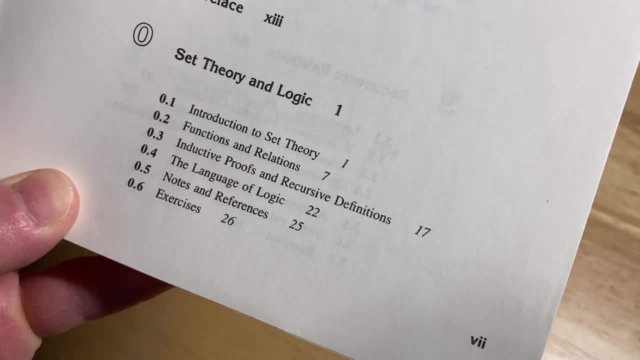 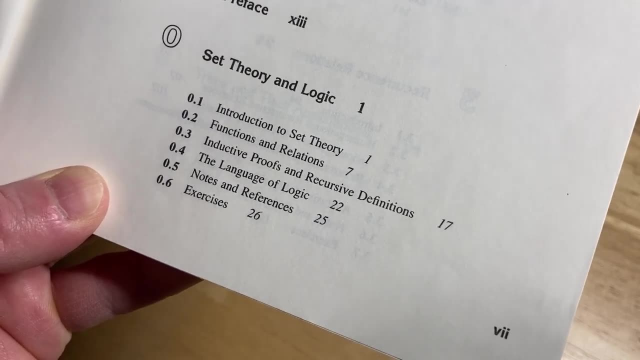 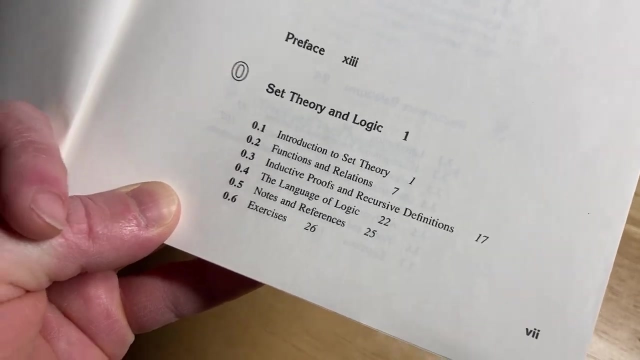 a little bit less expensive Set theory and logic. So it starts with the basic of sets. Most advanced math books start with set theory By the time you finish your math major. if you're a math major, you'll be an expert at set theory because you see it in like every. 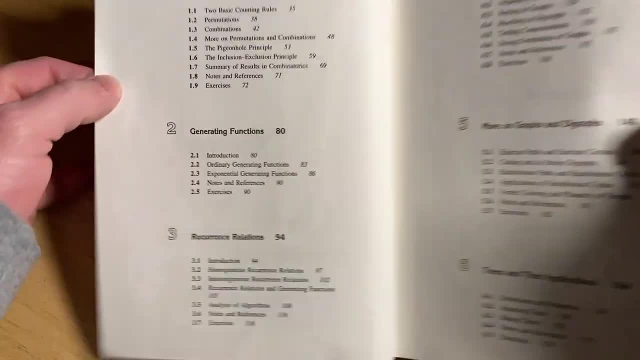 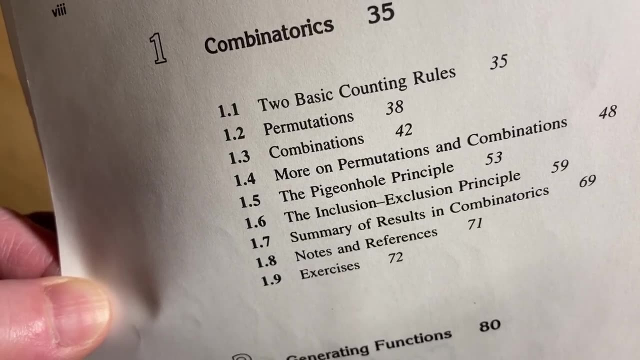 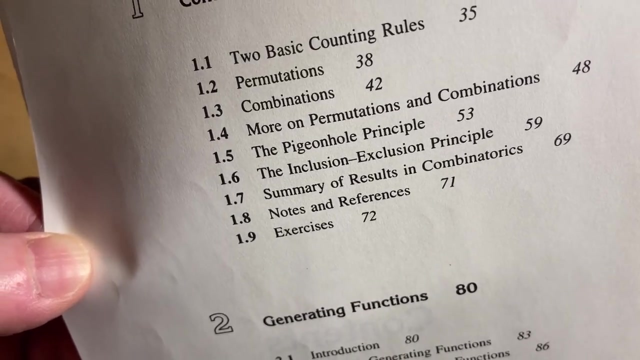 single class. Let's see what's on the next page: Combinatorics, That's the theory of counting. So it talks about two basic counting rules. Then we have permutations and combinations. More on permutations and combinations: The pigeonhole principle, The inclusion-exclusion. 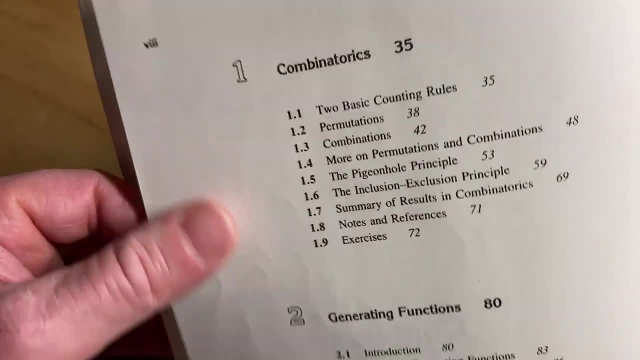 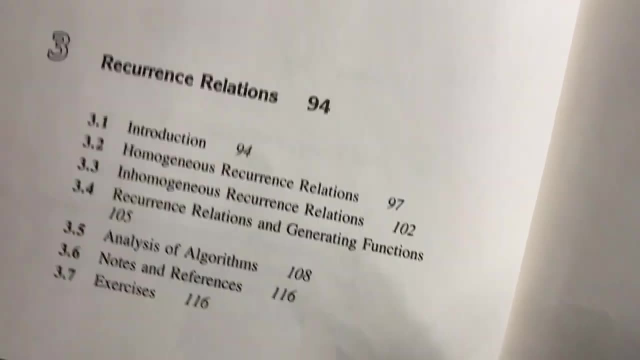 principle And some notes and references. I've read this entire chapter and I've read some of chapter two and some of chapter three: Generating functions, Recurrence relations. These are really cool. You can use these to solve counting problems and you can solve. 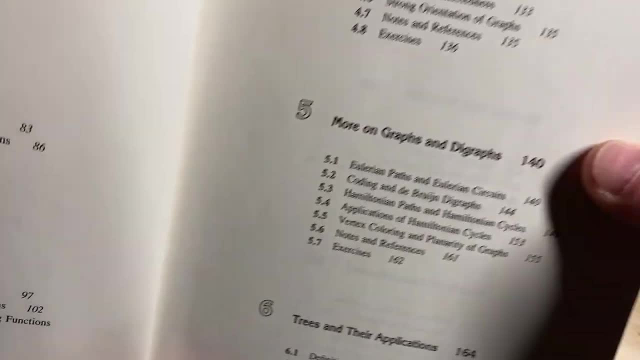 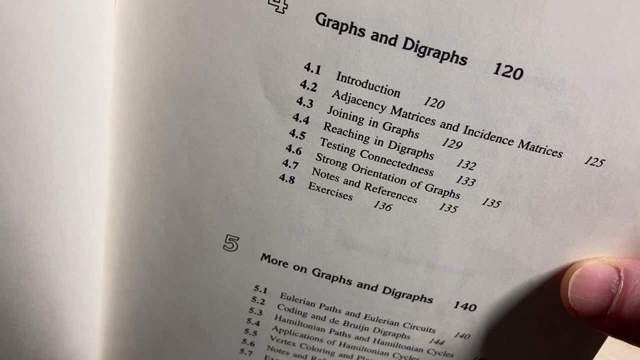 them in fun ways. algebraically. They're kind of fun to work through Graphs and digraphs. So you do get some graph theory, A discrete math book. you are exposed to graph theory as well. More on graphs and digraphs. 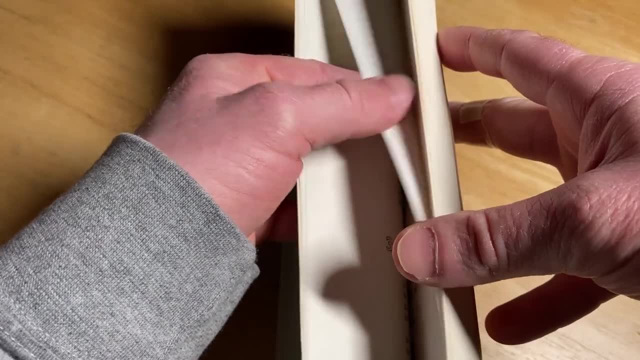 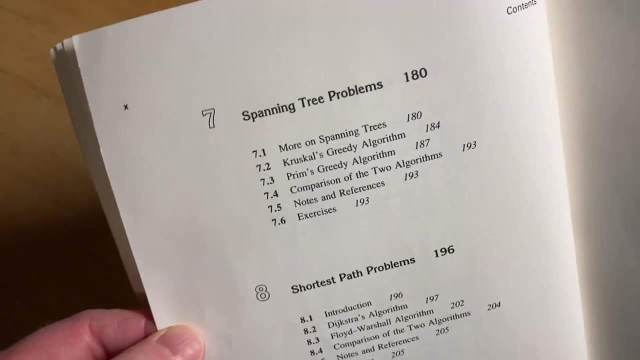 Trees and their applications. Typically, computer science majors are required to take a discrete math class. If you're thinking about going to college to learn computer science, then this can be something that you can have now and learn ahead of time: Spanning tree problems. 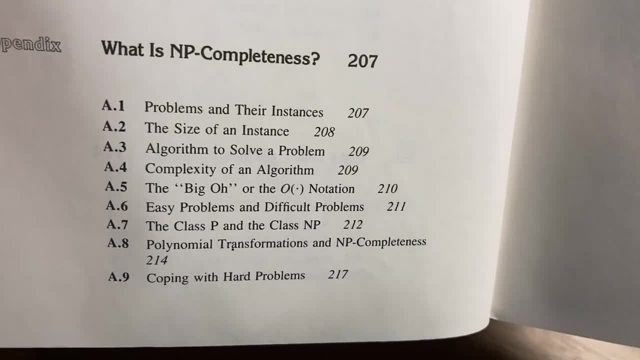 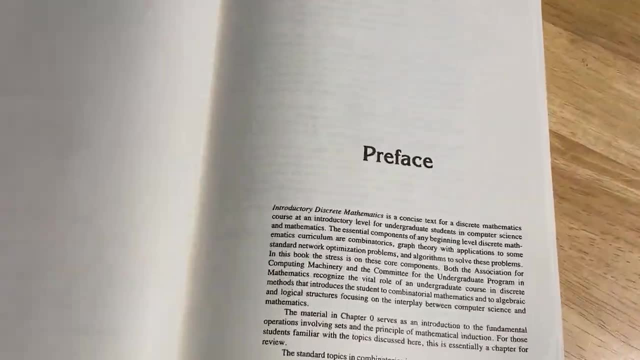 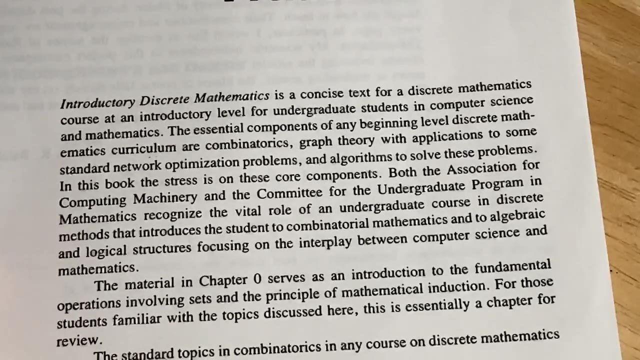 Shortest path problems? What is MP completeness? And then we have answers to selected exercises. So let's just take a look here closer at the book. Here it says some stuff about the book. Introductory discrete mathematics is a concise text for a discrete mathematics course at 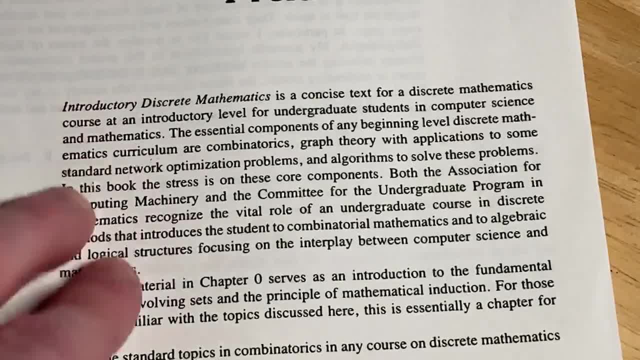 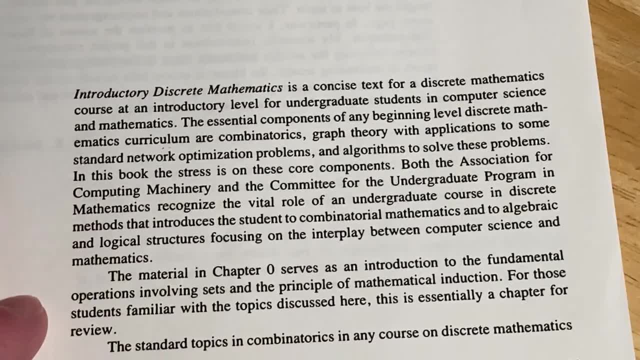 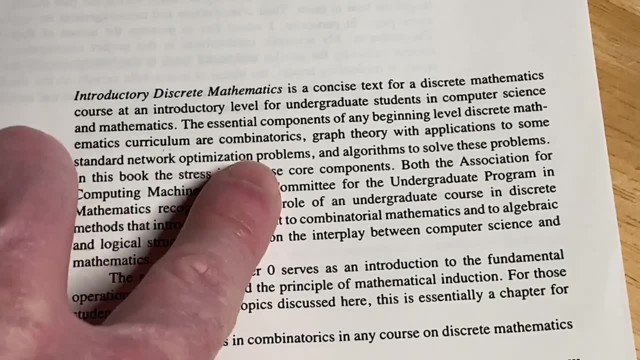 an introductory level for undergraduate students in computer science and mathematics. So there it emphasizes the computer science part. I was actually a double major for a while- computer science and math- And at that time I took discrete math, Eventually ended up switching to just mathematics- The essential components of any beginning. 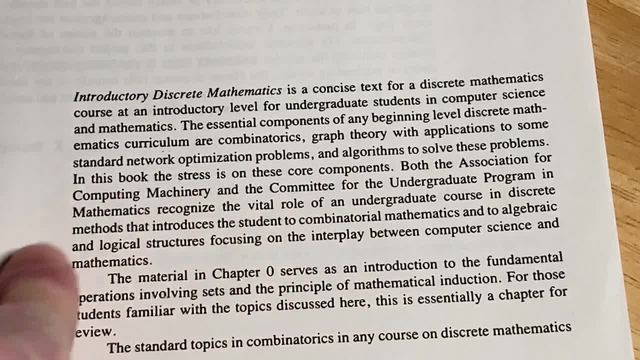 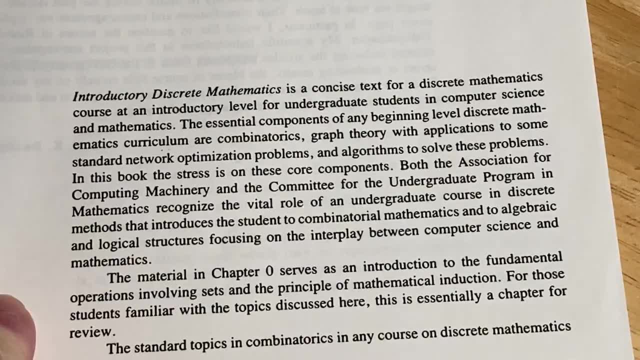 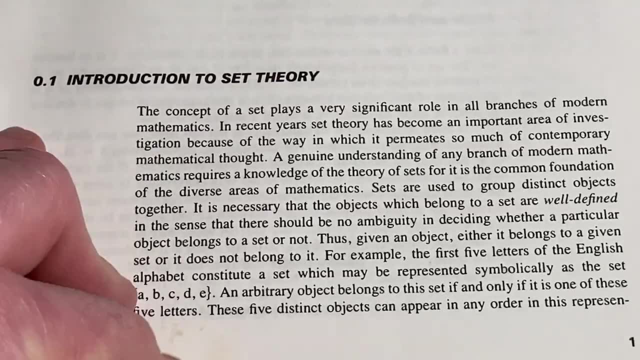 level discrete mathematics curriculum are combinatorics, graph theory with applications to some standard network optimization problems and algorithms to solve these problems. In this book the stress is on these core components- Cool. So it starts with set theory And again. 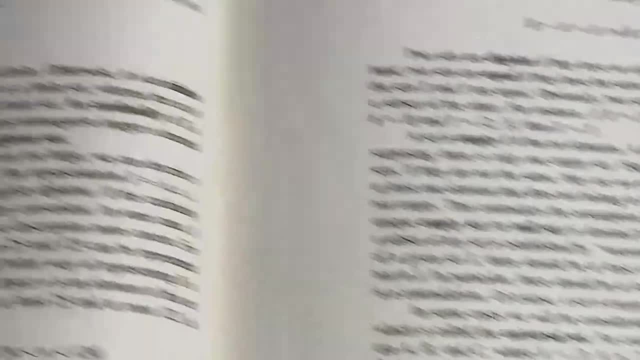 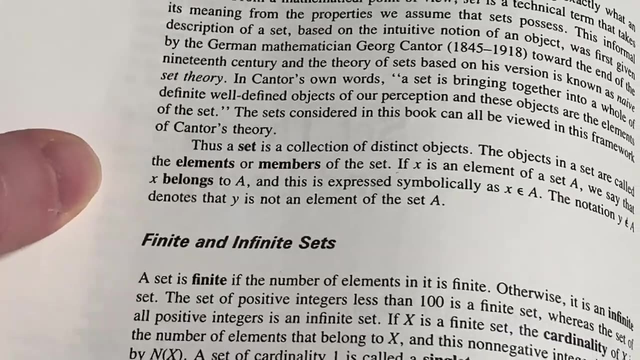 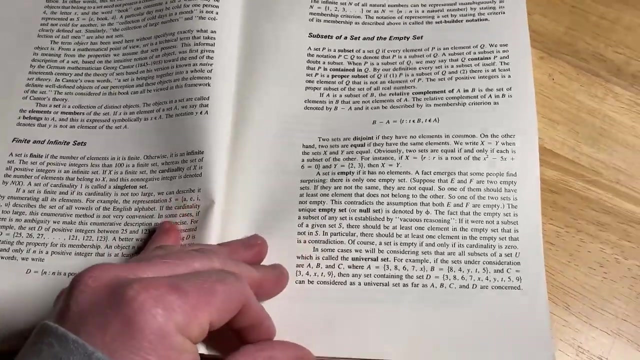 it's quite readable. Again, I've read a decent amount of this book: Finite sets. It goes pretty quickly. So every time you see a word in bold here that means that it's a definition. So it goes through pretty quickly. So, compared to some other discrete math books, it is a 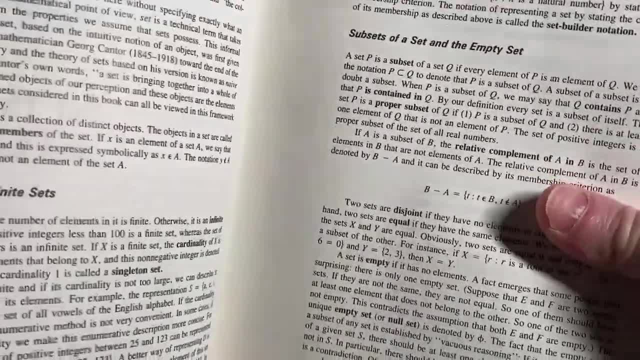 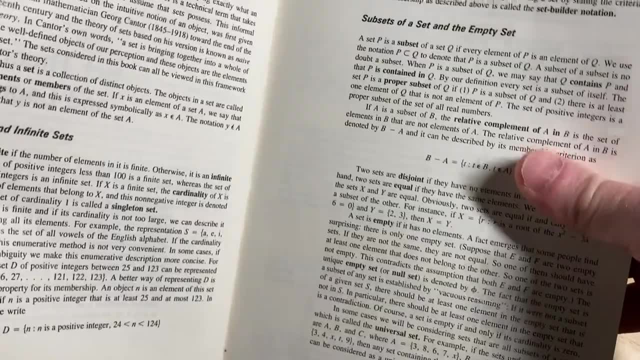 little bit more advanced. It's not like the easiest one in the world, But I like the size. I also like that it's a paperback because you can lay in bed and read it. With hard covers it's just they're not as good for bedtime reading. So as much as I love hard, 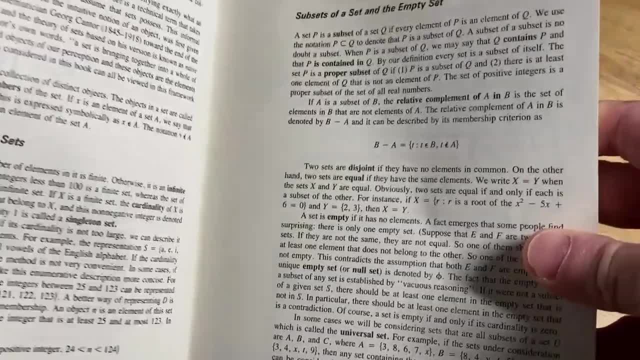 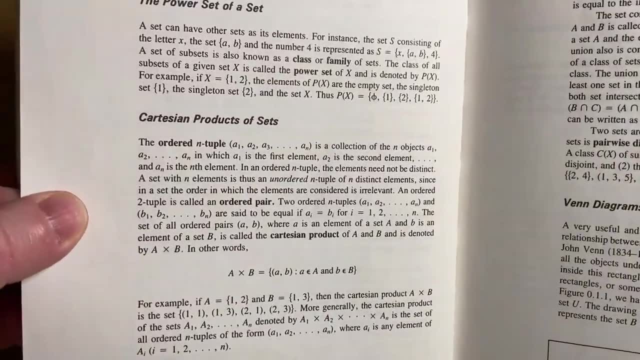 cover books. I prefer soft covers for reading before bed. It's just easier to lay in bed with a soft cover than it is with a hard cover book. Anyways, most Dover books, in fact all Dover books, are soft covers. The power set of a set, That's the set of 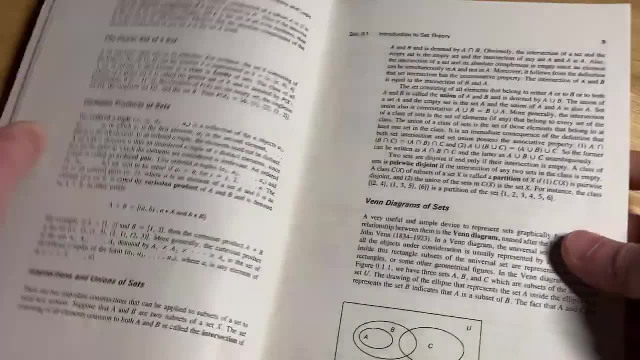 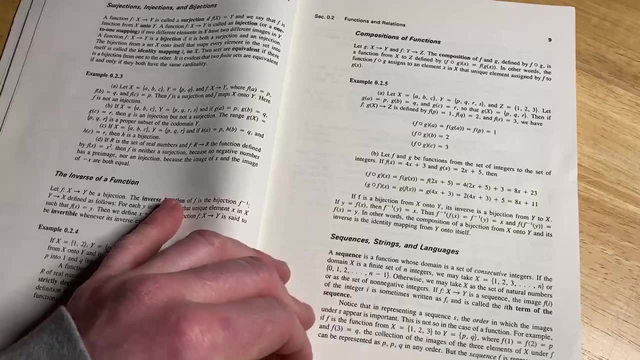 all subsets, Cartesian products. You see how quickly it goes through stuff. So it gives you a really quick review of set theory And you do have examples. So you see it does actually have worked out examples. These books are fun because you learn a lot of math. You can 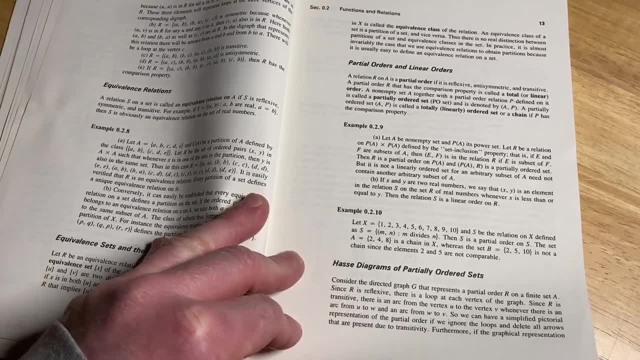 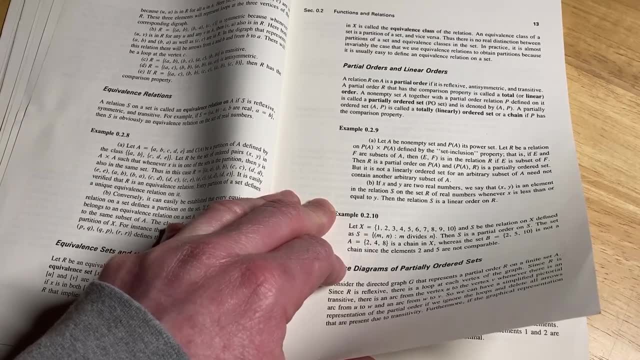 sit down and you can read for like 45 minutes and you'll learn something. I mean, you'll learn a lot. You don't have to understand everything, Like you're going to get stuck on stuff. My advice is: try to work through it And if you can't, it's okay to move on. 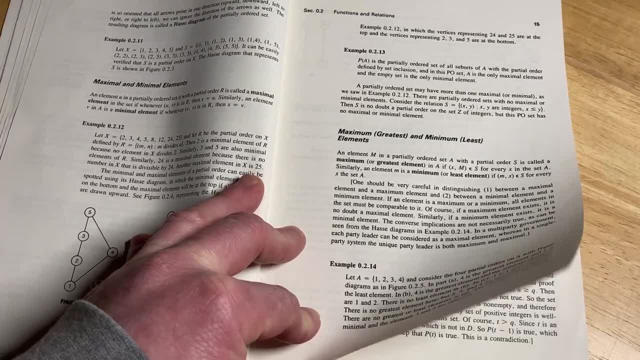 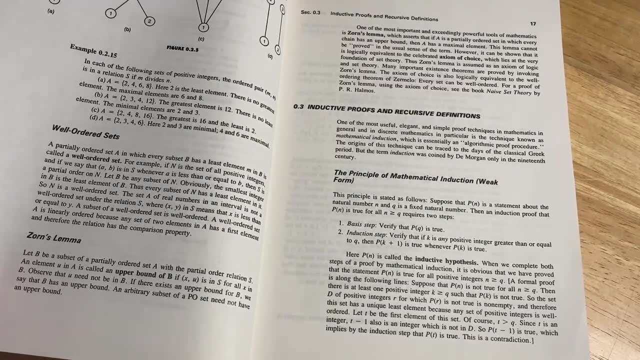 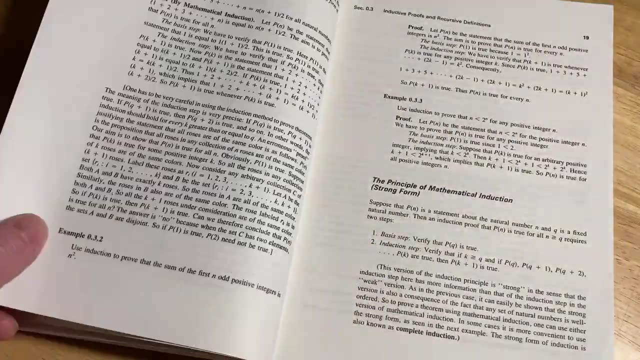 and just learn some more stuff. Try to maximize your reading time. Try to learn as much as possible in the time that you've allocated for your nighttime reading or daytime studying. Ooh, Zorn's Lemma- Max Zorn, He was a famous mathematician. Zorn's Lemma is named after 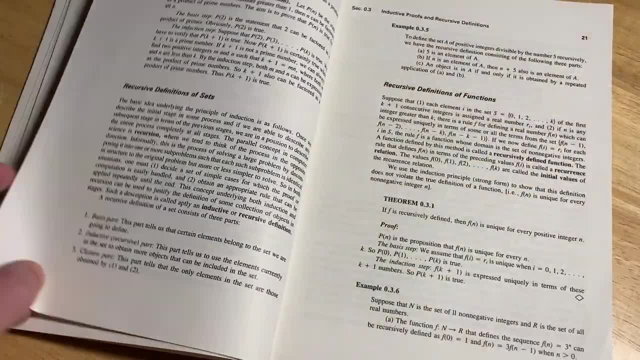 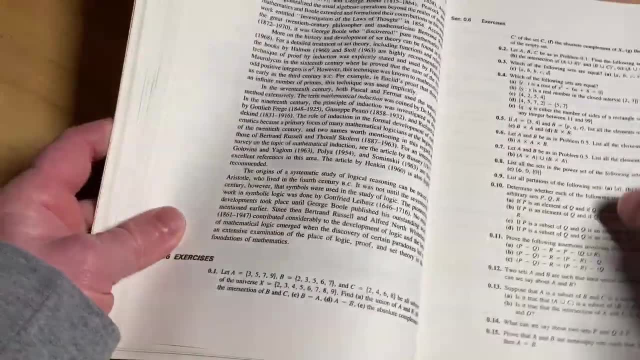 Max Zorn, Some induction stuff. Then if we go to the very, very end, we have exercises, So the exercises don't appear until the actual end of the chapter, which is okay. I mean you get some, some reading and examples. 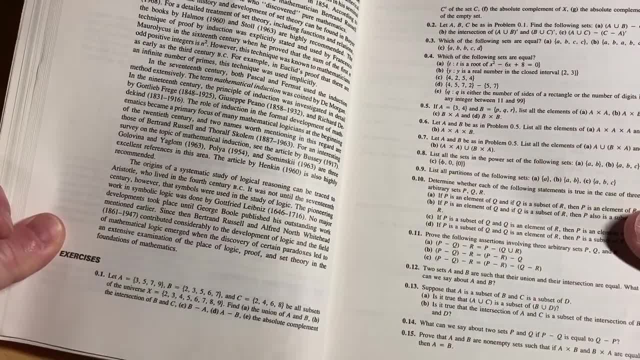 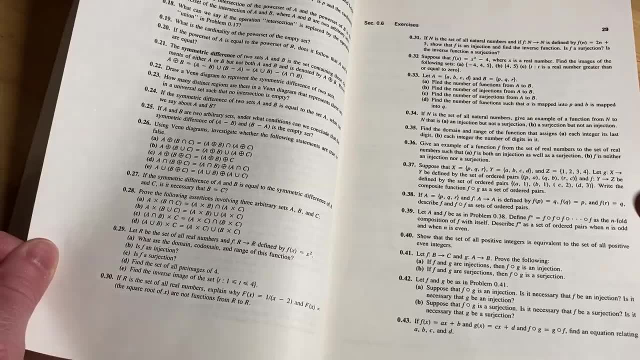 So you do read quite a bit and then you get some exercises. The exercises are really fun. I've done some of them. I think they vary in difficulty- You've got some easier ones and you've got some harder ones as well- But it's just kind of like a fun book to work. 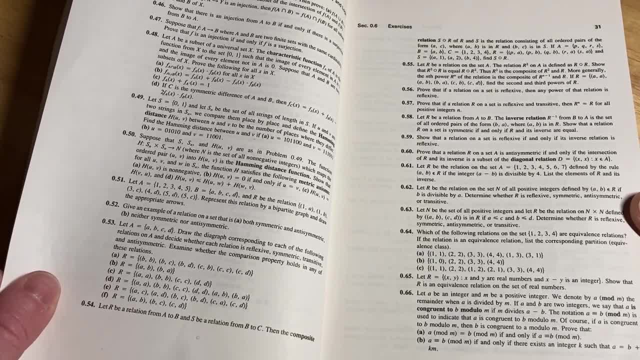 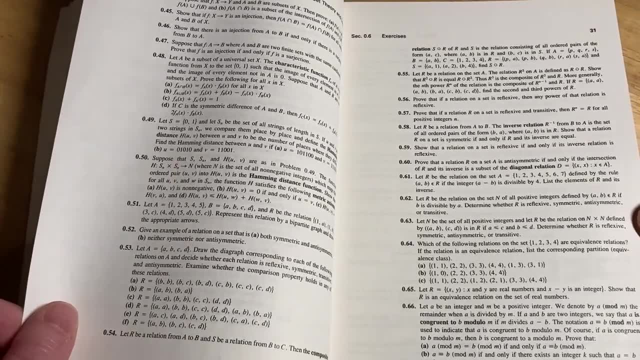 through. This is one of my favorite books, even though I don't think it's the easiest discrete math book. i think the easiest one might be the one by ep and if i remember, i'll try to leave a link in the description, but that one's way more expensive than this one, this one and 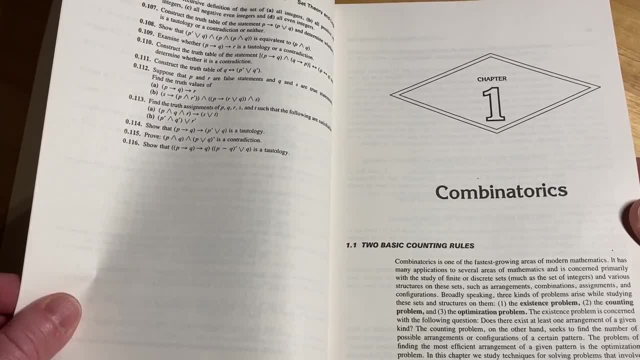 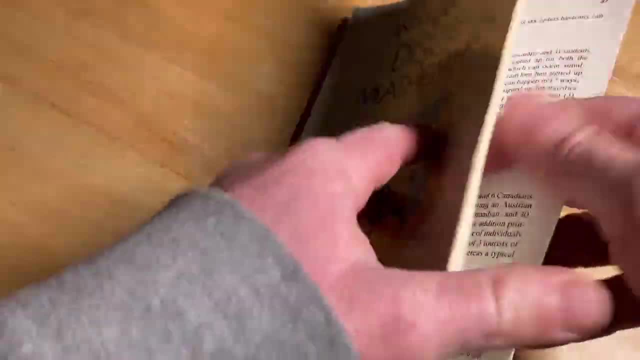 that one's hardcover. it's huge. i don't really think it's suitable for like bedtime reading. this is something um i like for bedtime reading. i know i keep saying that, but that that's what i think about when i see this book- some bedtime reading, because i've read it before bed. um. 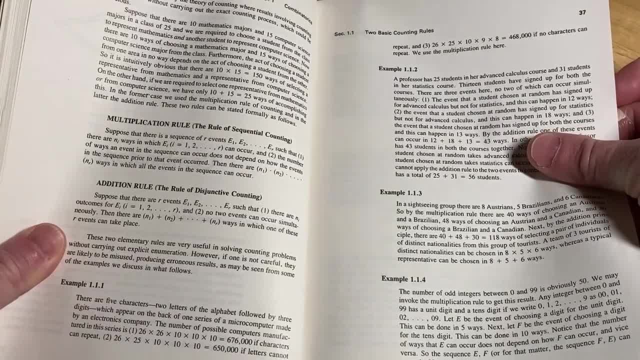 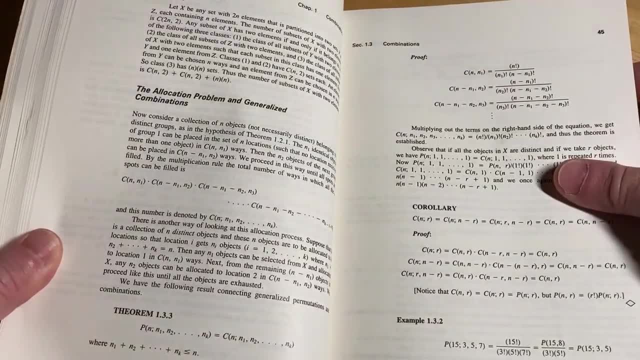 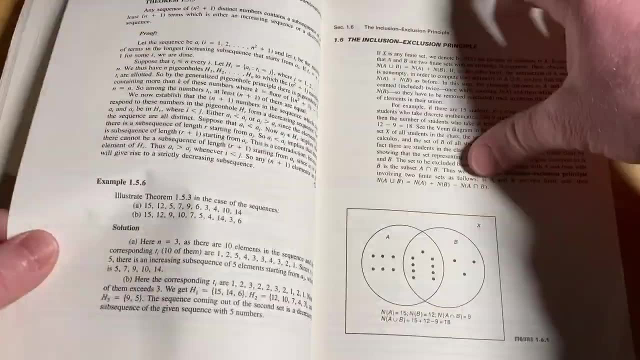 several times and also you can take it with you. one time i was at the mechanic, i took this book with me and i sat there for two hours. uh, and i read this book for two hours straight. so that was kind of a fun experience sitting in a mechanic shop, learning mathematics. and if we go to the end, 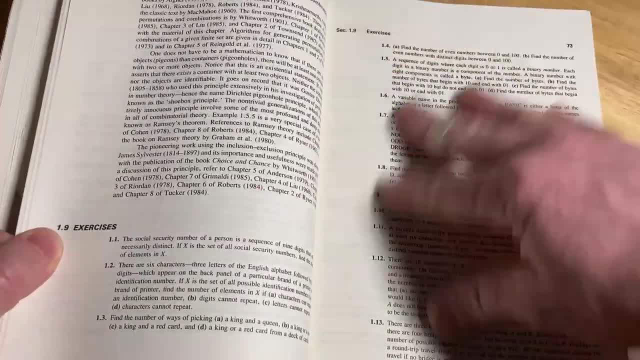 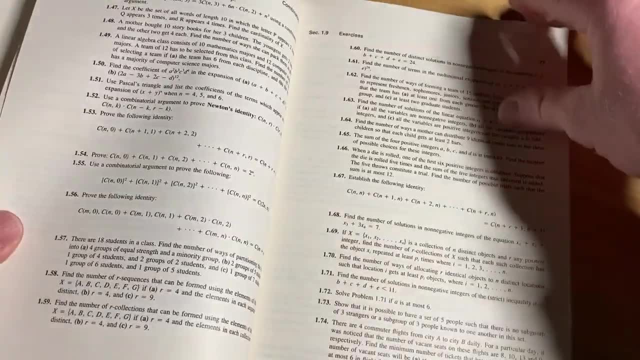 of chapter one. let's look at the exercises there. you get tons of exercises uh as well over here and the exercises do have answers. so let's look at that. wow, look at all these exercises. right, i just want to sit down like right now and start doing math problems. i think i might actually after. 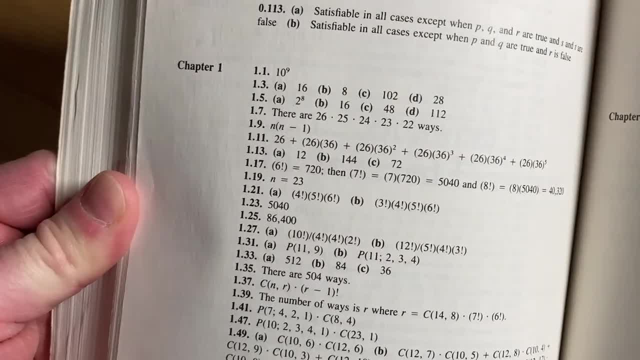 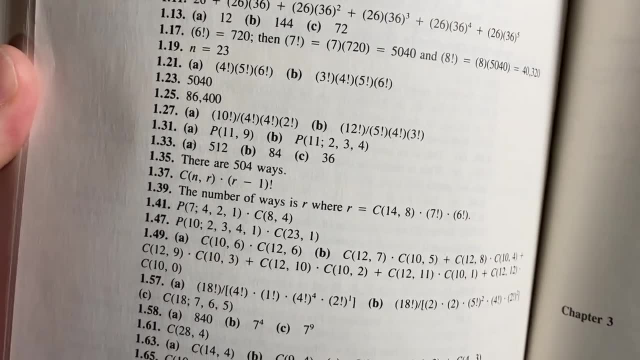 i make this video. i might sit down and read a little bit of this. you see, you have answers to the odd numbered exercises, which is really quite nice. oh, these are really fun. it's a different type of mathematics, by the way. so if you, if you don't know much about discrete math, it's a different way of thinking. 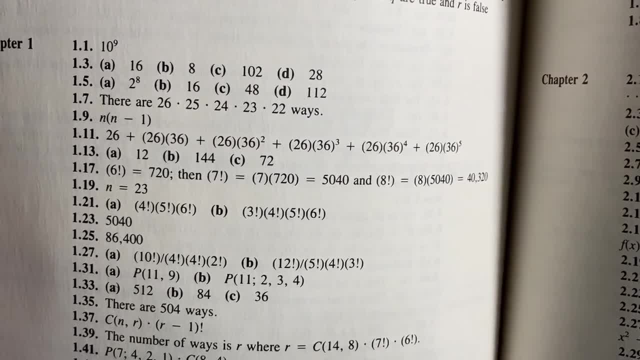 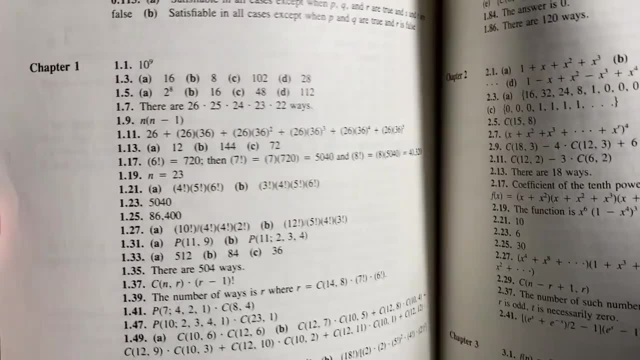 uh, and i think that's that's a good way to put it. i remember when i was in statistical theory- uh, which is a course which covers counting, probability, uh, and statistics- our teacher said that you had to think differently for the probability of the answer to the question. 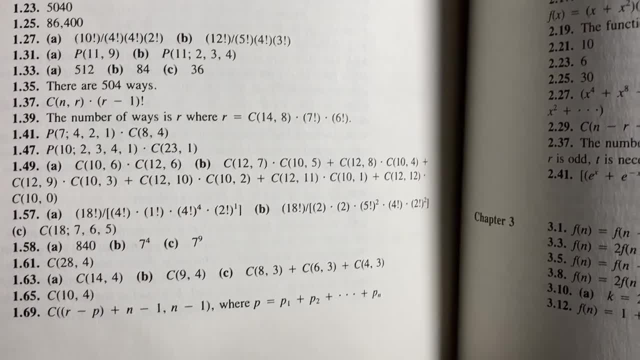 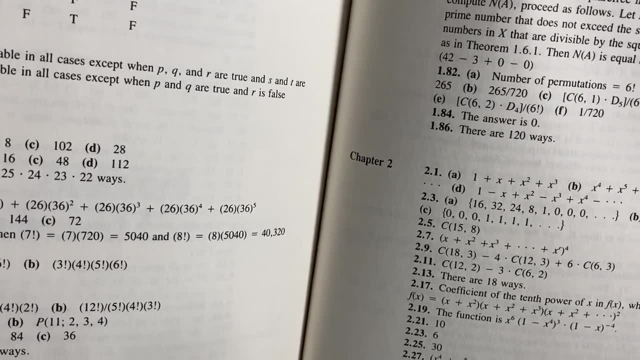 so it's a different way of thinking. and he was right, he was 100 correct. it is a different way of thinking. now it looks like it's more than just the odds. you got some even numbered answers here as well. so balakrishnan does say selected exercises, so that could be just the odds. maybe. 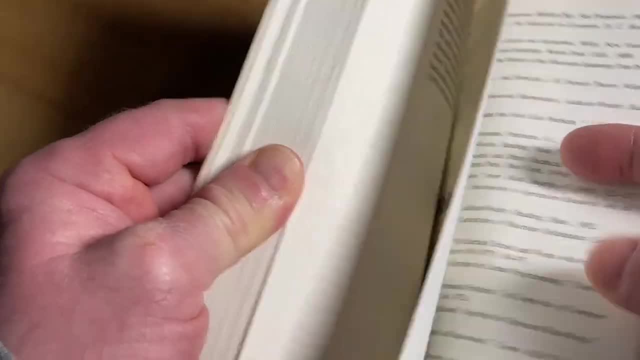 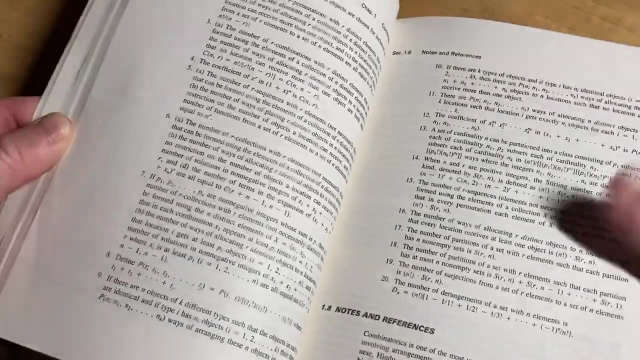 the odds and some more. um, it's hard to tell. you've also got some references here. you've got a bibliography. it's got to give it a whiff here. ah, what a great book. so this is a book that is a very worthy purchase and again, i will leave a link in the description. 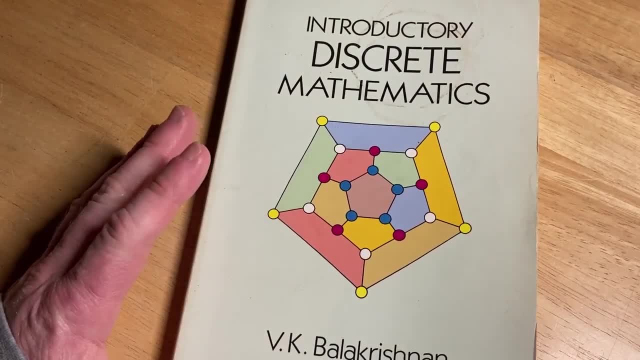 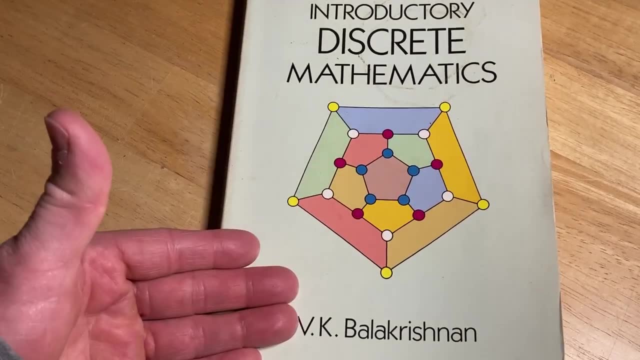 in case you decide you want this book just for, like bedtime reading or or doing math or as a supplement, whatever. i think it's a good book worth owning and belongs in everyone's library. bk balakrishnan is a great author. he has other good books. this one is introductory, discrete. 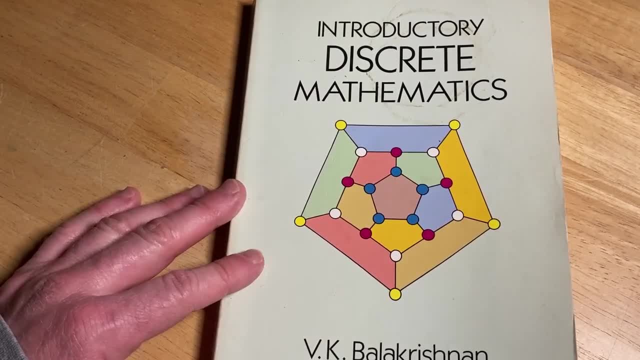 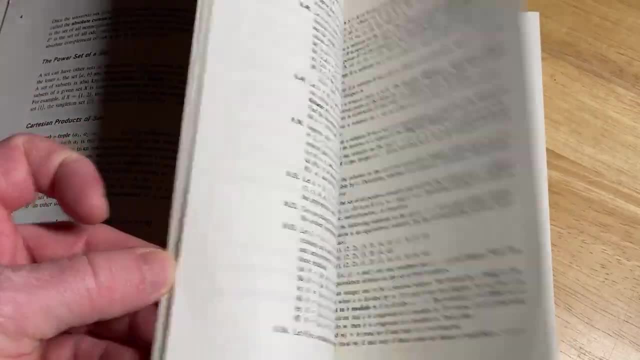 mathematics and i highly recommend it if you want to learn mathematics. by the way, i do have courses. they're on my website, mathsourcercom. they're actually on the udemy platform, but if you get my courses, please use the links from my website, for two reasons. first of all, i'm going to 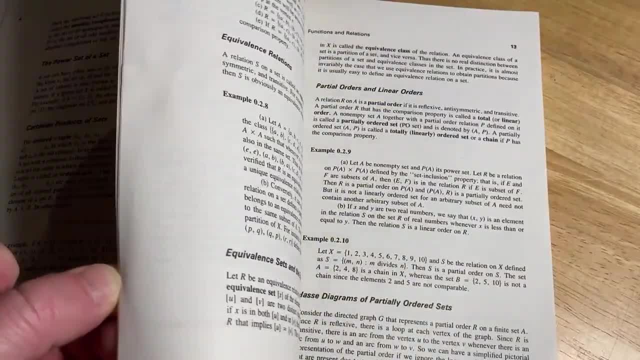 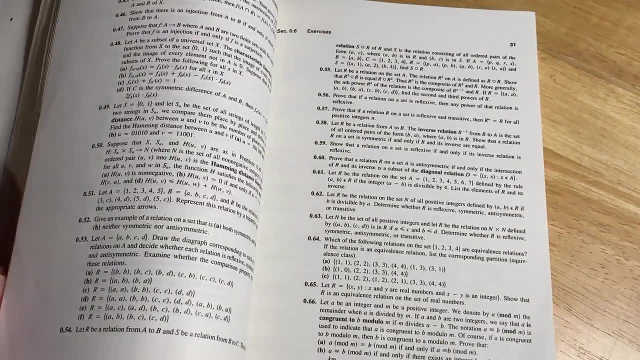 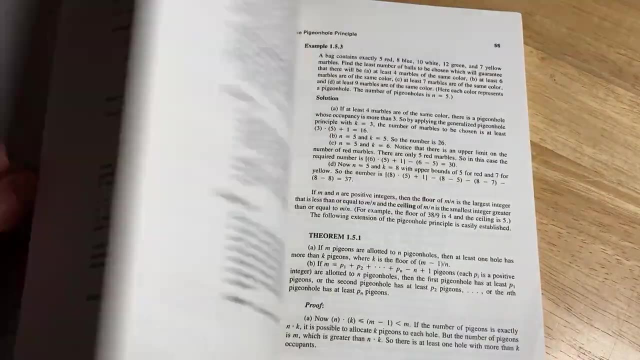 one, it helps me a lot because otherwise udemy takes pretty much almost everything. they take a big chunk, it's a lot. and two, i've lowered the price of all of my courses to the bare minimum. so if you use my links from my website, i'm pretty sure you're always going to get a very low price. 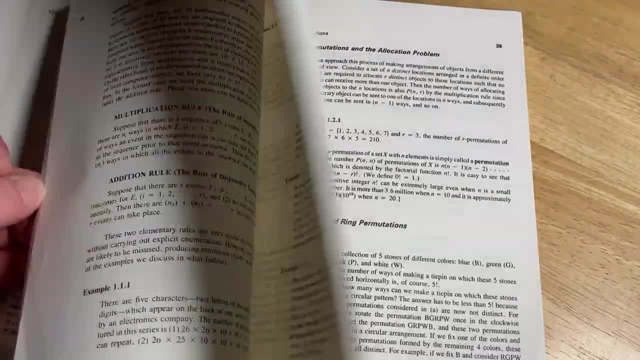 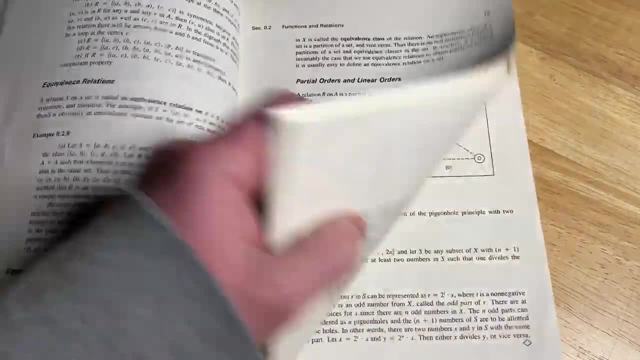 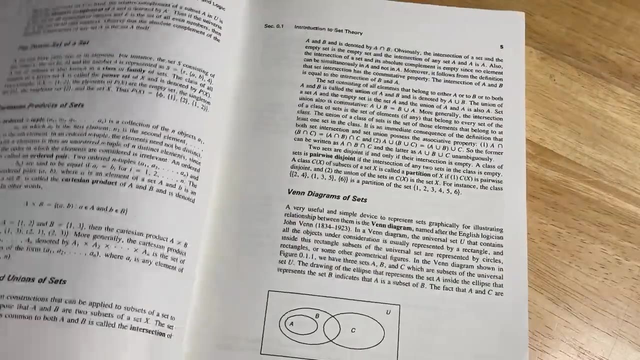 because i set the price at like the lowest level it let me set it at. so again, it's mathsourcercom or just freemathvidscom, but check it out. i've got courses on algebra, calculus and proof courses, abstract algebra, advanced calculus, etc. so i don't have a discrete math course yet. 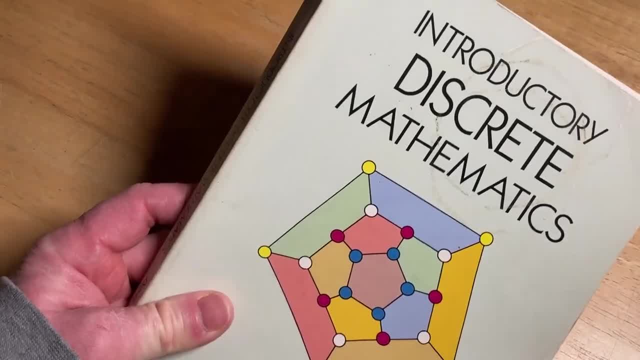 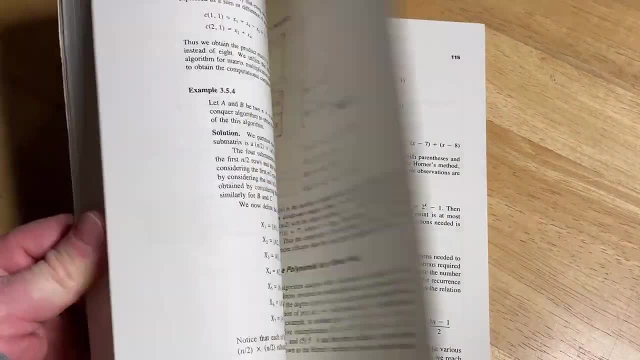 someday maybe, but yeah, check it out and if you found any value in this content, feel free to hit subscribe if you want to. also, i always forget to mention this, so i should. i do have another youtube channel. it's called the internet sourcer. it's undergone some name changes. i think i'm going 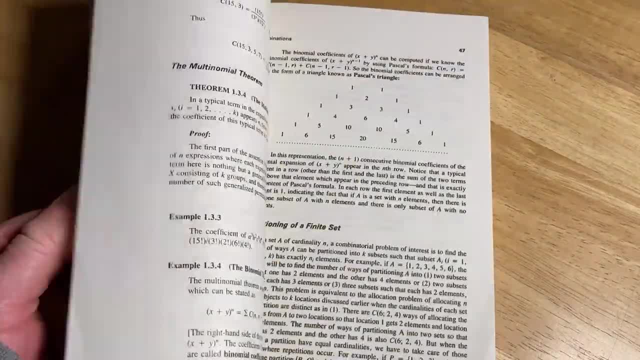 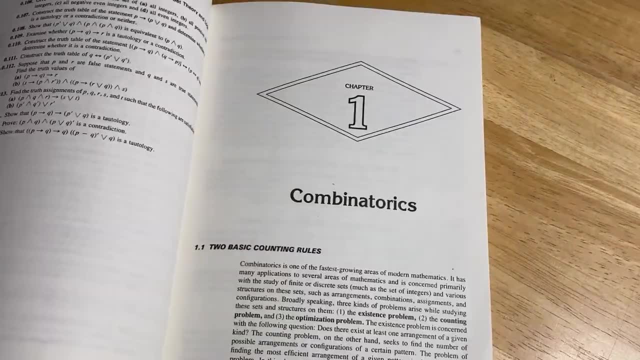 to keep it at the internet sourcer, so it's kind of like more in line with the math sourcer. i post all kinds of stuff. they're just random stuff, so anything goes on that. it's like anything goes channel. so check that out if you want to follow me for more content and stuff like.